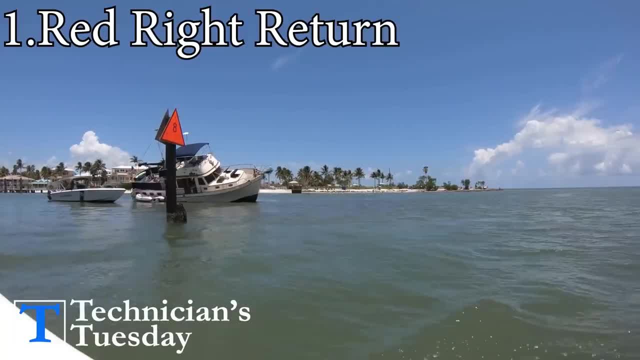 Remember these five phrases: Red right, return brown brown, run aground. green green, nice and clean. white white you just might. and blue blue, run on through. These phrases will help keep you from having a horrible experience while on a boat. This week's contest prize is something that will. 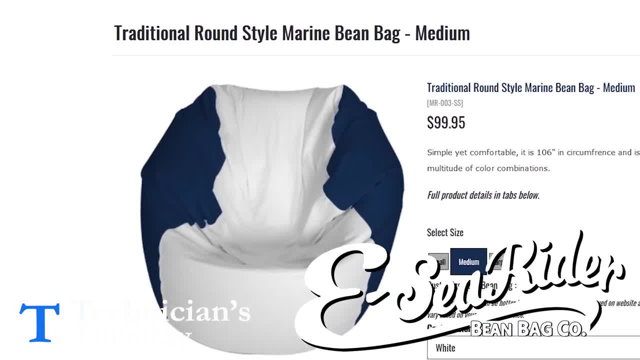 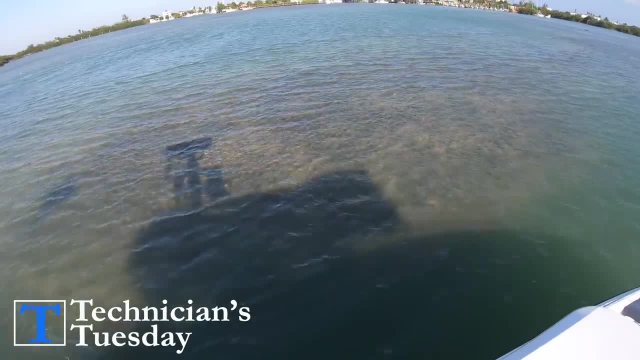 definitely give you a great experience on the water, because this week's prize is an Easy Rider beanbag from Easy Rider here in Florida. When doing any boating anywhere that you are unfamiliar with the water, the first thing you need to do is to check on the tides and at what times they are. 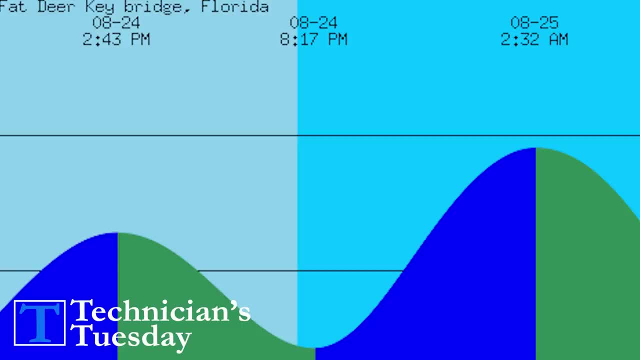 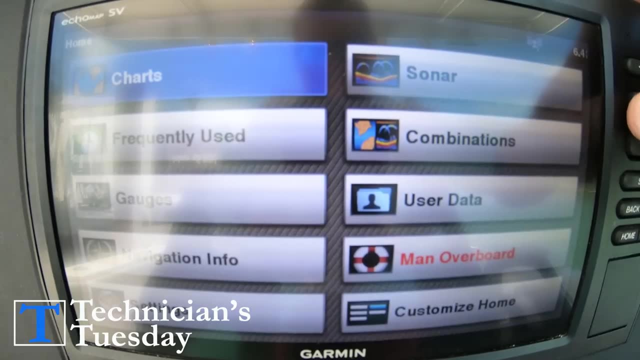 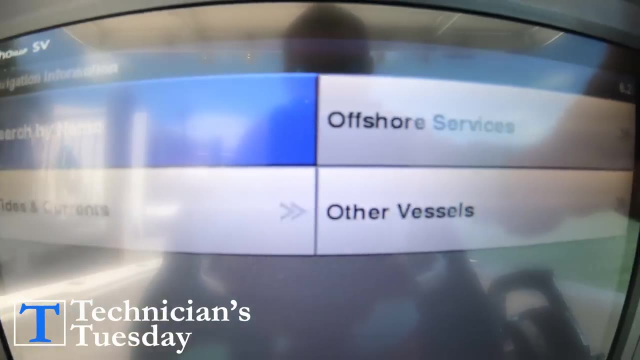 changing. Which is a cool thing with most newer GPS chart plotters these days is that you can go into the information section and they will actually have tides and current charts. that will even let you check on the tides for wherever you are planning on going. 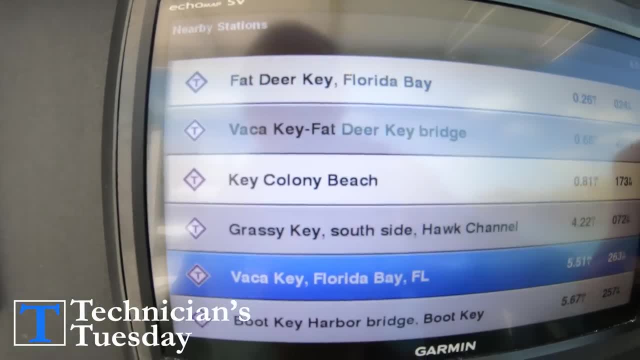 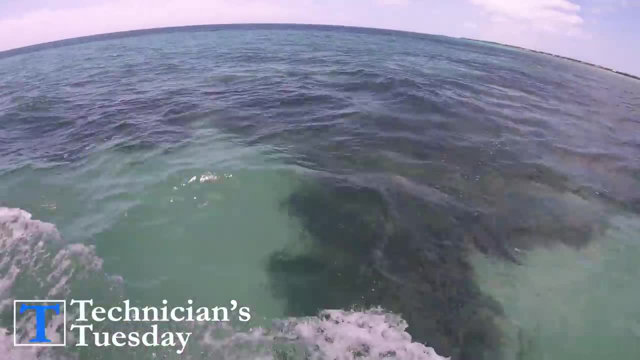 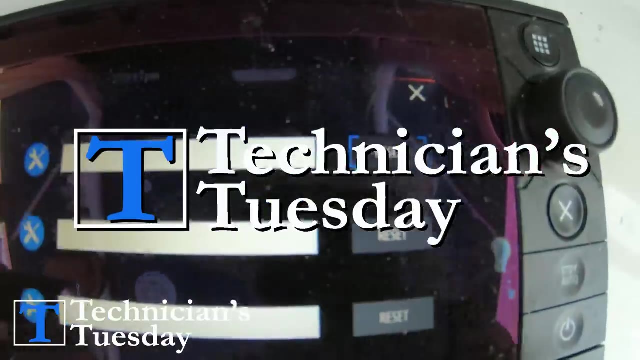 This is important because tides can swing great distances depending on where you are located, and if the water depth drops, say, four feet, you might find yourself hitting ground when at another time you wouldn't. Yes, this is Technicians Tuesday, but because of the COVID-19 outbreak. 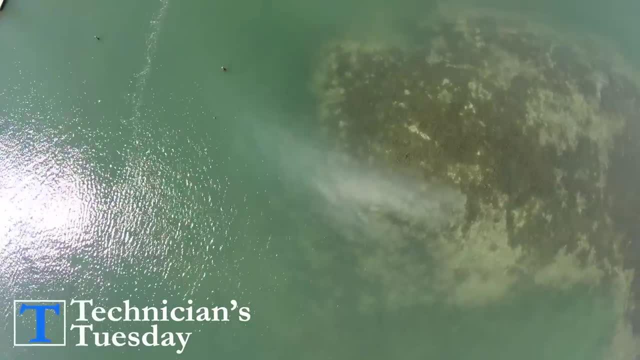 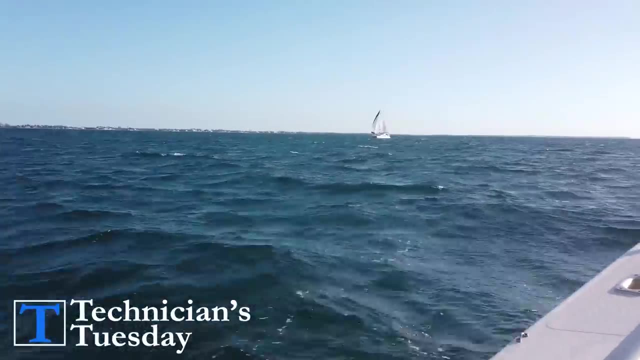 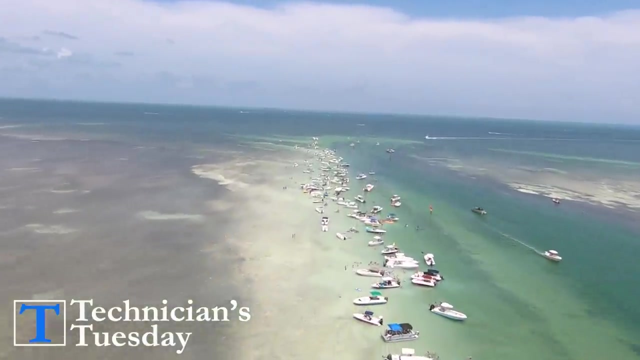 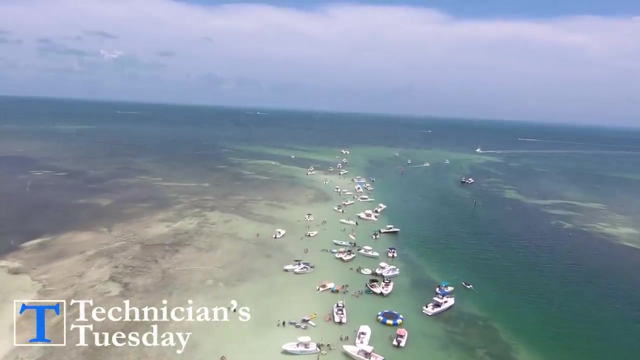 we're going to change the content up a little bit this week and we'll look at the technical aspect of how to read the water. So what exactly these phrases mean is the basic foundation of being able to read the water and know how to avoid running aground whenever there aren't any markers available to show you. 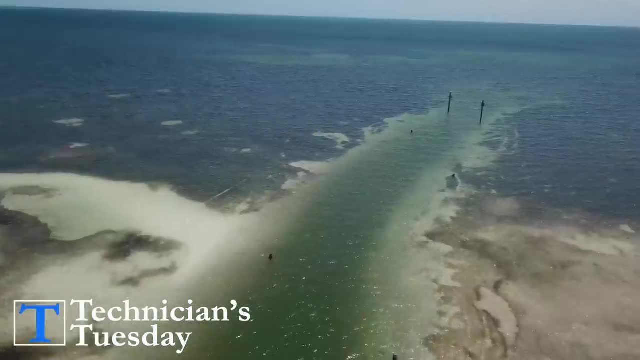 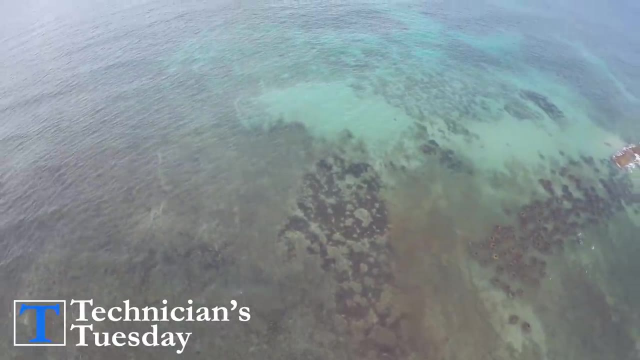 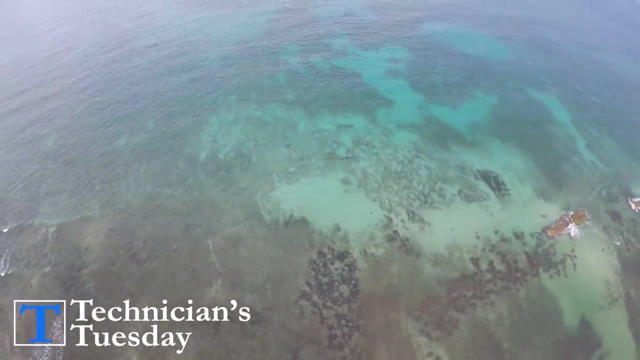 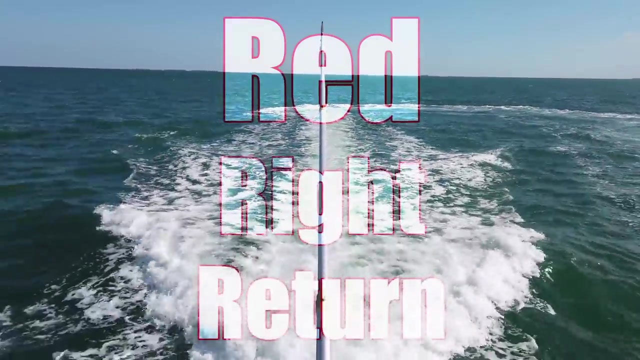 what is going on while in the water. You'll notice that each phrase reference has a specific color. knowing the water color is going to show you more about depth of the water than you might otherwise think. The first phrase of red-white return: this isn't a reference to the water color, but 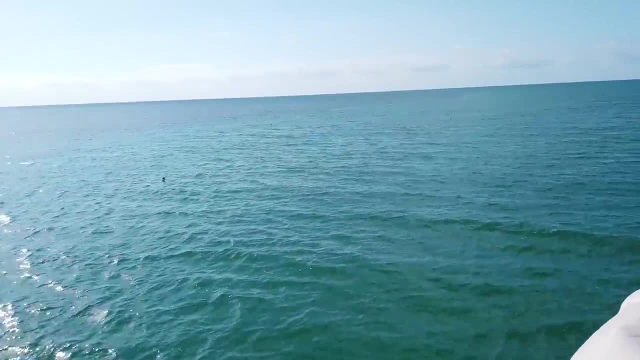 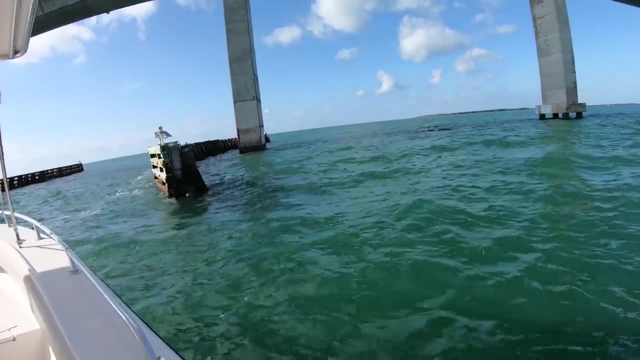 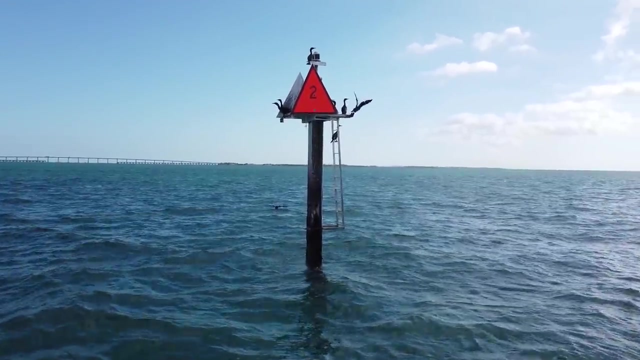 what it is is the most commonly known and general term for channel markers that mark where a channel is and where to avoid. This simply means that if you are returning from a larger body of water, like the ocean, then when you enter into the channel, that red marker is going to be on your right and 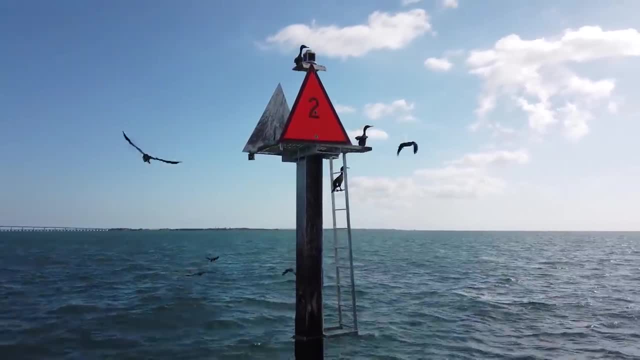 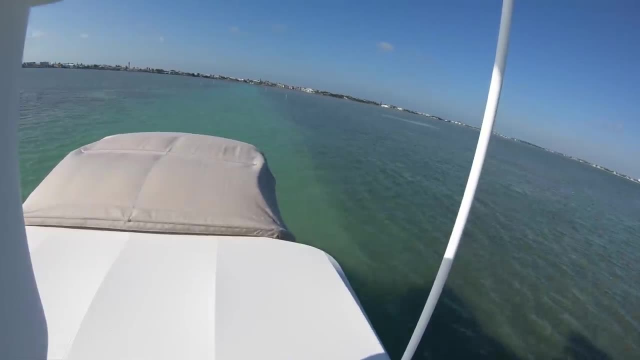 you will generally find them to be a red triangle with an even number on them. That is a saying that every boater should know, but the bulk of today's video is about looking at where you are going and being able to tell if it is shallow or not before hitting. 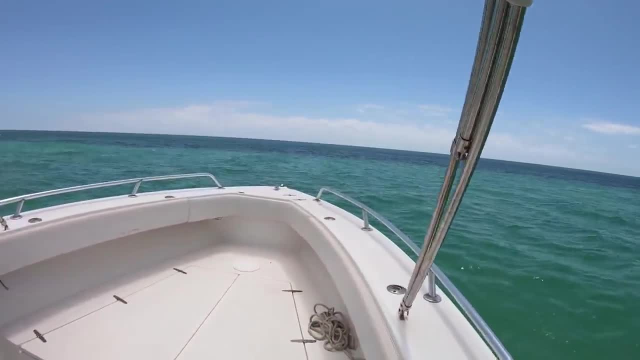 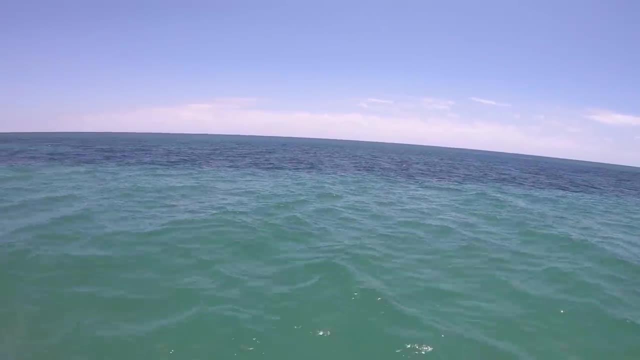 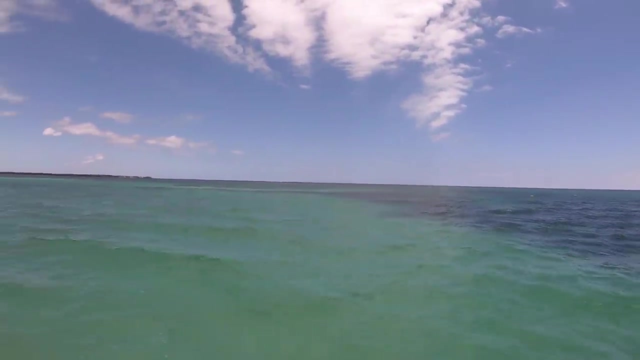 the ground, which- this is the basic rule of thumb- you want to slowly creep up on wherever you are going, Ok, And have a spotter, or physically get up to the bow and look into the water to see what's going on. And we've got another video that we'll link to in the description about docking and 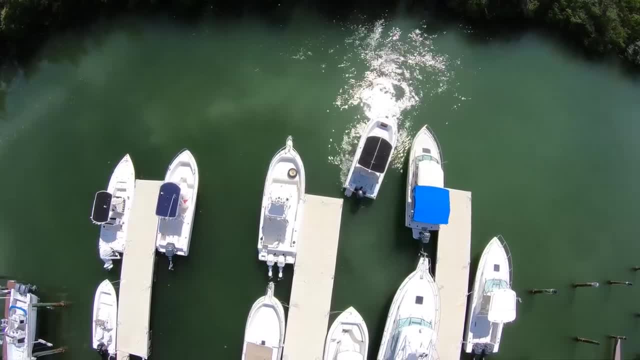 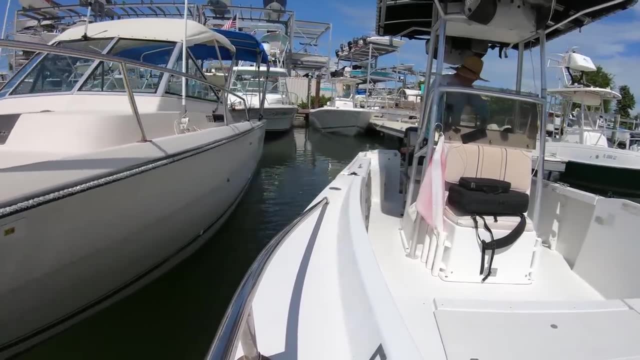 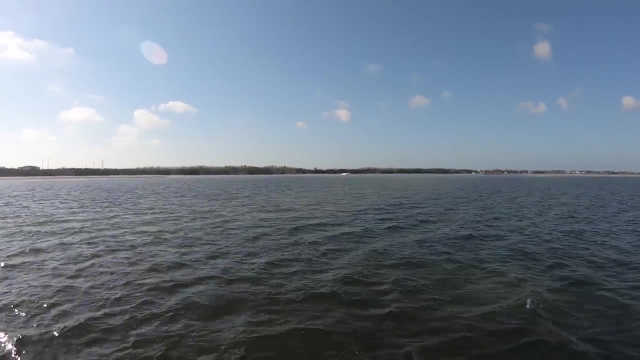 how to handle a boat. that will give you some great pointers to instantly improve your boat driving skills, to give you the confidence to be able to slowly creep up into wherever you are trying to take the boat. This is what you have to do whenever there aren't any markers and if you remember. 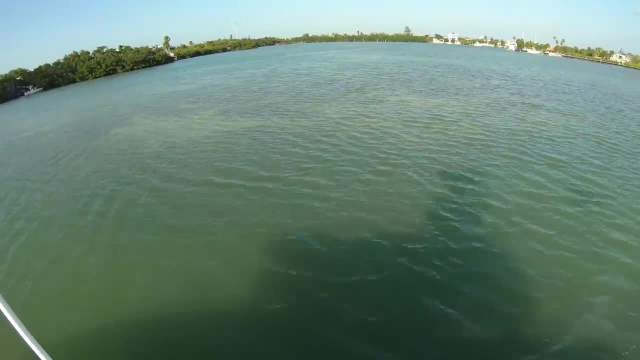 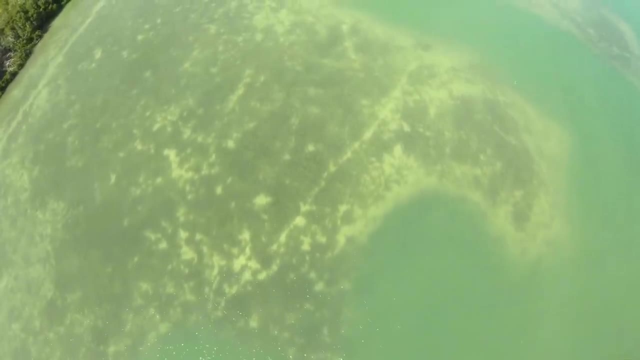 how to do that, then you'll know that whenever you see a dark color of water or a brownish color, that the water there is extremely shallow and you are basically looking at the ground. Now, depending on the time of year and your geographical location, the water color can. 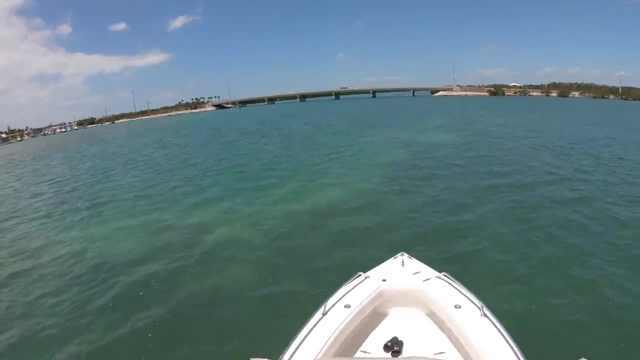 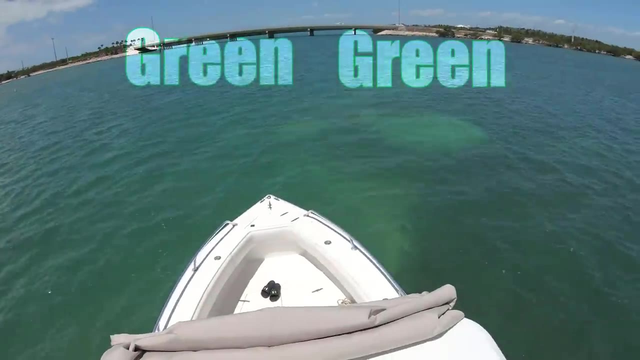 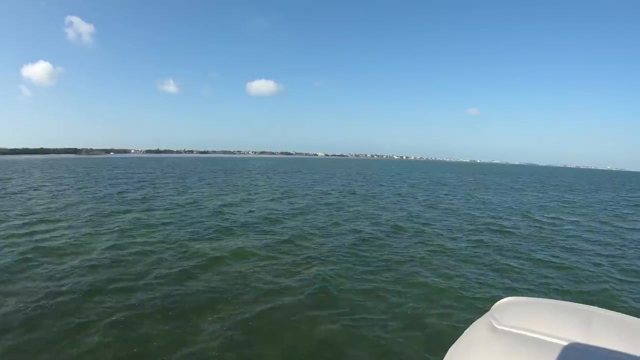 change to a point, During the winter months or when it is cooler out, the water color is actually going to be a greenish color, which is why the next phrase is green, green, nice and clean. Ok, Thanks for watching. Then, whenever it is warmer outside and we are in the summer months, the water color 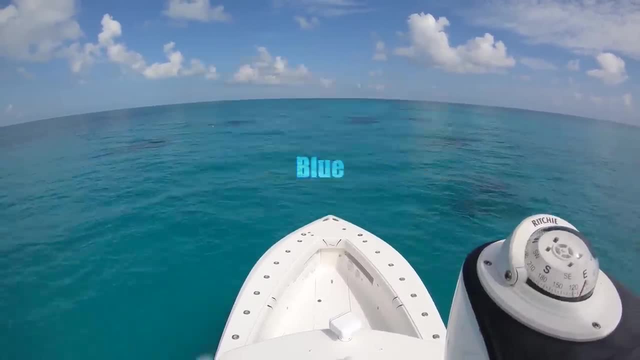 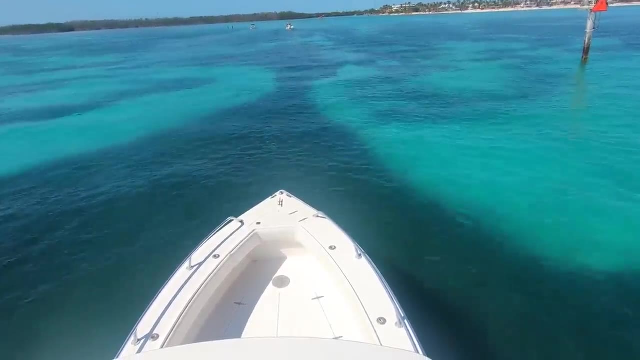 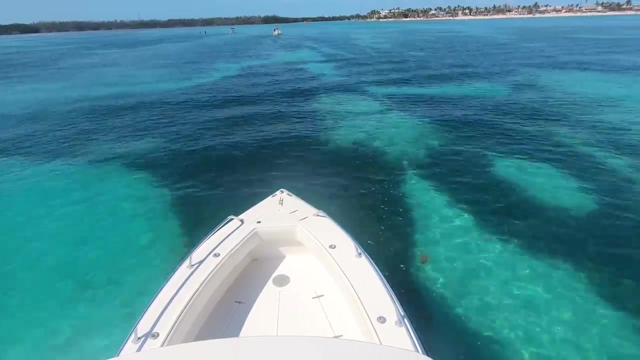 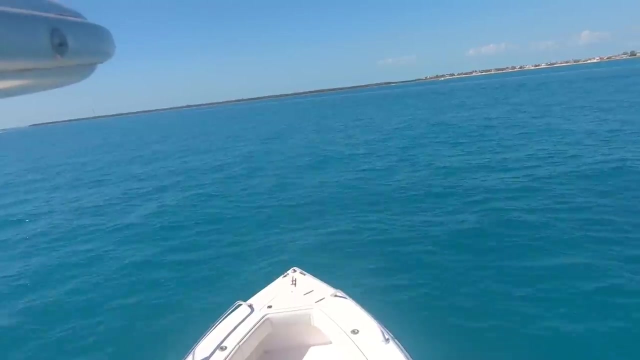 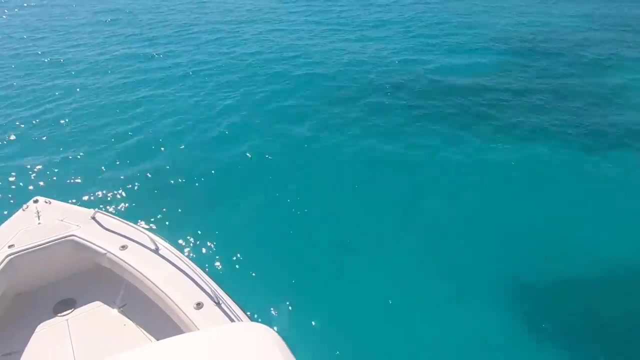 is going to be more of a bluish color, giving us the blue blue run on through phrase. This is also dependent on the location of the sun. Whenever the sun is directly overhead, it is pointing straight down into the water, which is generally when you will get those beautiful teal blue pictures that you see. 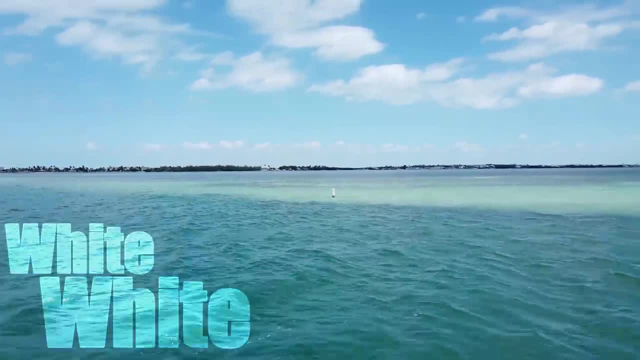 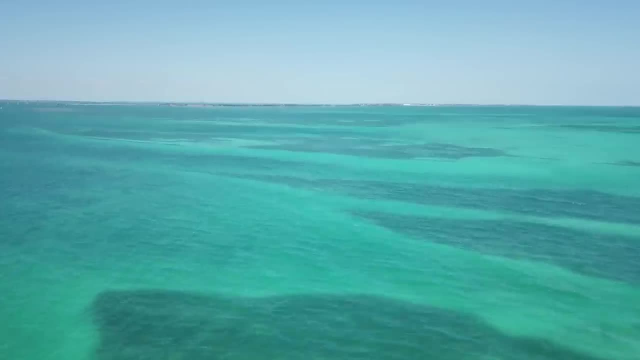 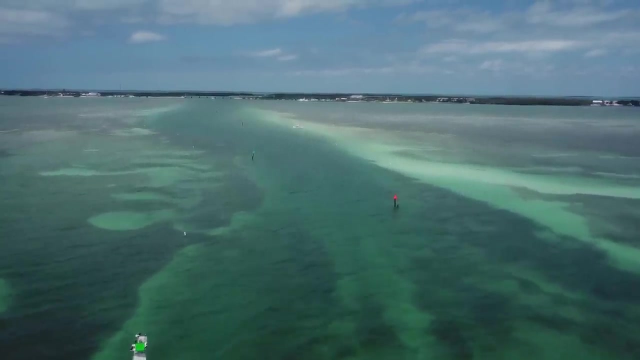 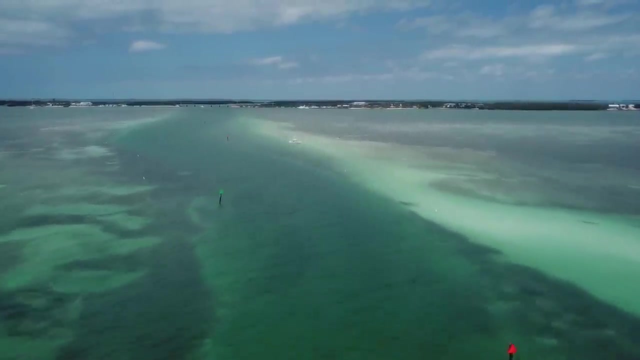 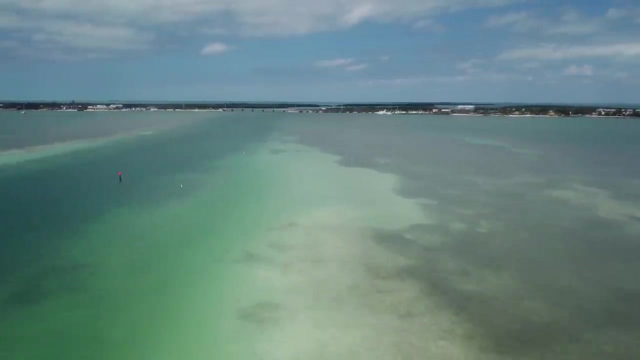 posted all over the place. Our last phrase is white, white, you just might. and this phrase is to remember to watch out for sand bars. Whenever you see clear, clean, almost white patches in the water, these patches are of sand. Whenever it gets low enough, you will see white sand exposed.